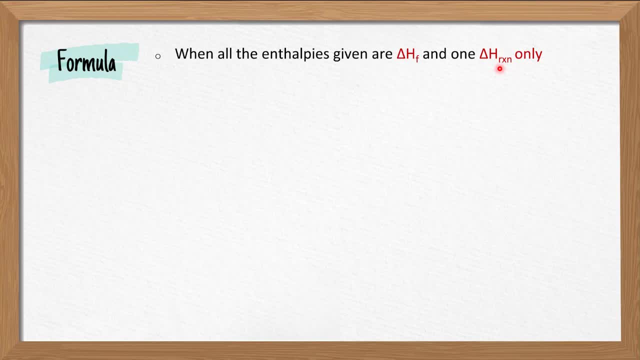 in that question you only consist of enthalpy of formation. These enthalpy of reactions can be bölt Bam birth At night. so a few enthalpy of formations and only one enthalpy of reaction, and make sure that all the 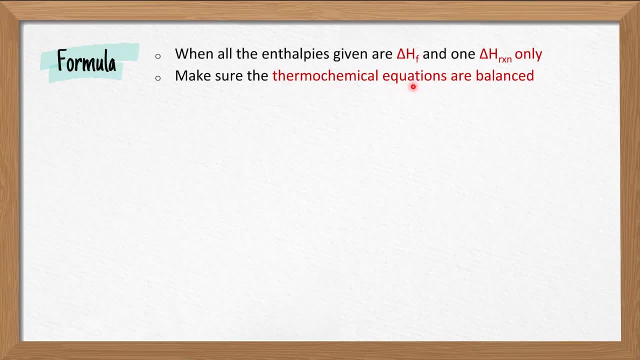 thermochemical equations are balanced Because we need to use the stoichiometry ratio to apply this formula. So we have: the enthalpy of reactions equals to the sum of enthalpy of reactions equals lo rough, equal results. So we have to close this formula because we have flipped it and checked that this is an international integral discussion factor And that's why we cannot use this formula. So we just need to �midade. 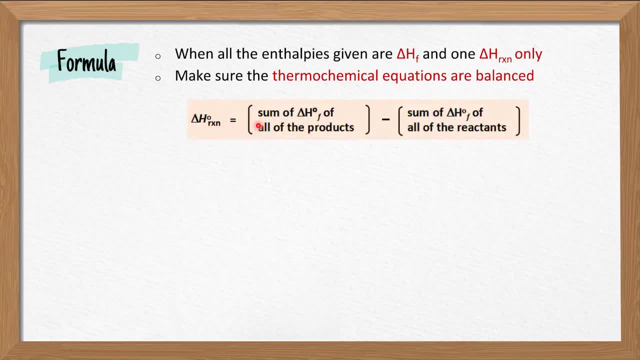 we have the enthalpy of reactions equals to the sum of enthalpy of formations of all the product, minus sum of the enthalpy of formations for all the reactants. So product minus reactant. So of course, from here you need to have a balanced thermochemical equation. 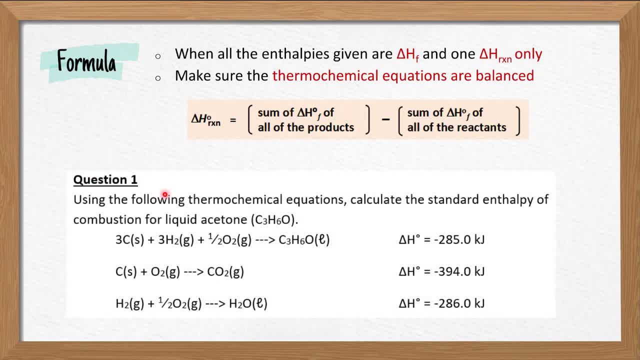 So, given in the questions, one, using the following thermochemical equations, calculate the enthalpy, the standard enthalpy of combustions for liquid acetone C3H6O, and you're given a series of thermochemical equation. So in this case you need to find: 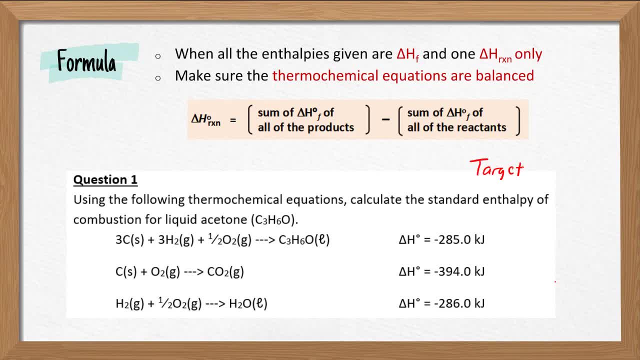 the target. Target is what we want and what is the questions asking about. So, standard enthalpy of combustions. write down the symbol: standard enthalpy of combustions. You can also write this one as the reaction, So this one refer to the enthalpy of reaction. 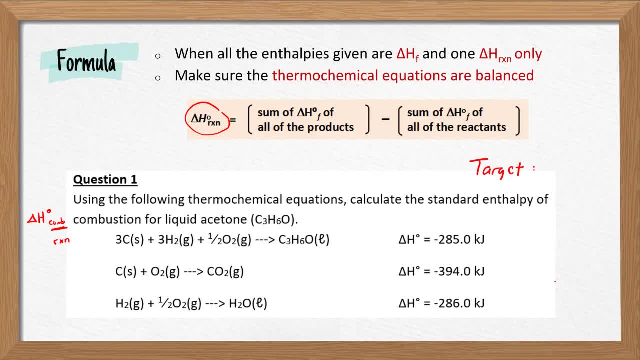 And this target. you need to have the equations For this target. write the equations So I will show you in the next slide And let's interpret the equations given over here. As I told you just now, you need to have only one reactions- enthalpy of reactions- and a few enthalpy of reactions. 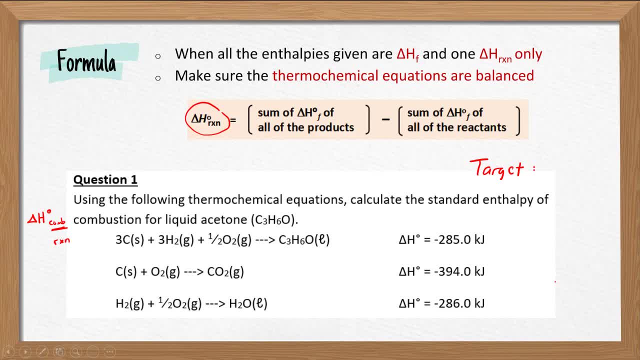 So here is your enthalpy of formation. So, according to the definitions, when one mole of the compound is formed from its element under the standard state. so this carbon hydrogen, oxygen are all the elements at standard state. So this enthalpy. 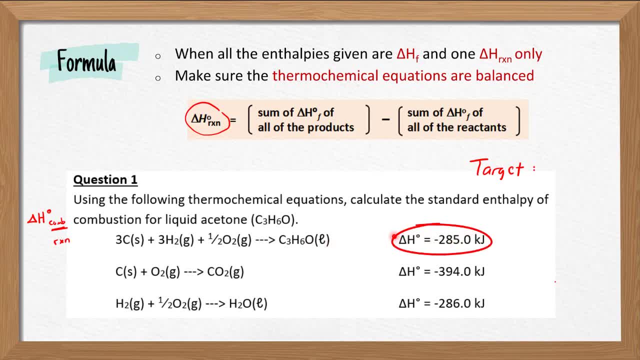 refer to the enthalpy of formations for C3H6O. The next equations: when one mole of carbon dioxide is formed from its element under the standard state, so this enthalpy refer to the enthalpy of formation for carbon dioxide, CO2.. The last one: when one mole of H2O is formed from its element. 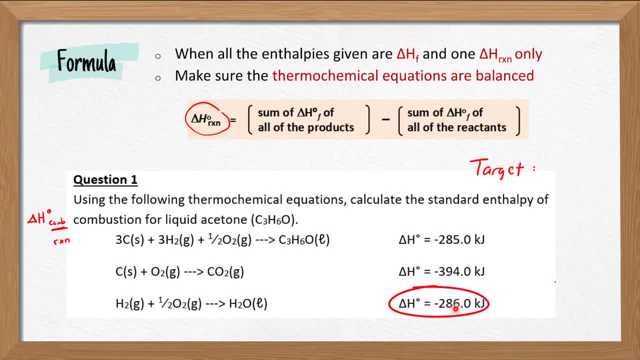 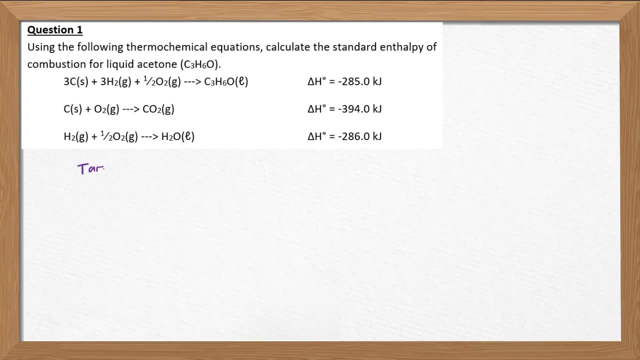 at the standard state. so the last one refer to the enthalpy of formations for H2O. So you may write down over here: these are all enthalpy of formations. A moment for just clinic, very brief. So for this question, start off with your target. You need to identify what. 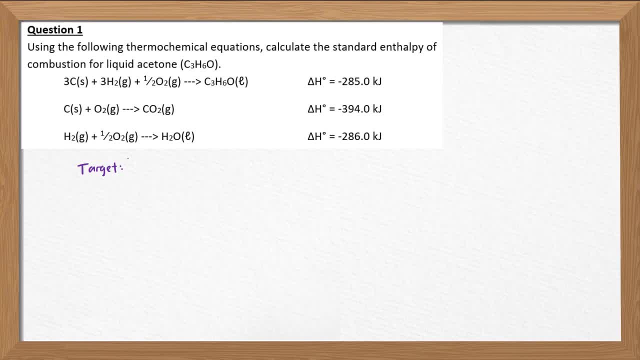 is your target. So target is what you need to answer for the questions: Thermo chemical equations which, referring to the combustion Bombs, reactions of acetone. So C3H6O is your target and the best hormone that is composed of shadows of. 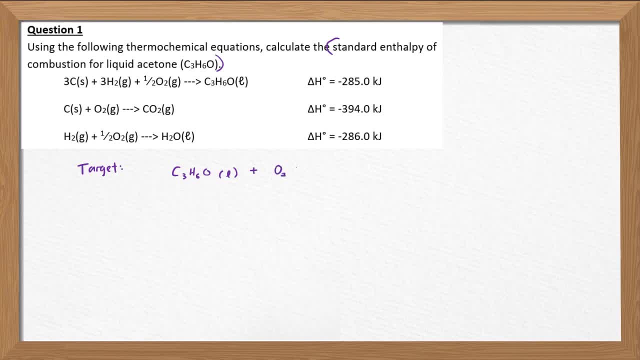 carbon dioxide gas, the injection of oxygen gas. you can visualize the come When this is commuxed in oxygen gas. it will produce carbon dioxide gas disseminates in the gas waste to make carbon dioxide acid acid a real reaction to oxygen. These 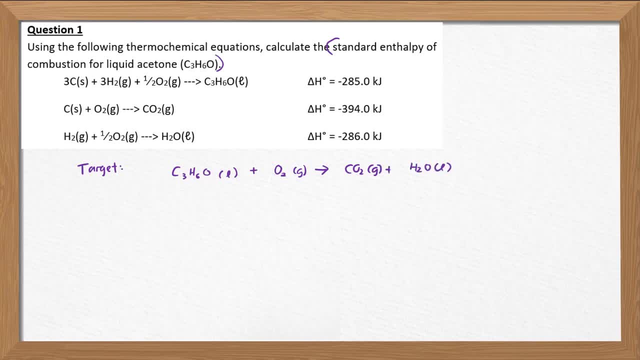 liquid for the product, because this is a hydrocarbon, so the product will be co2 and h2o. so if, according to the definitions, when one mole of the acetone is combusted, okay, you will release how many heat. so this is what we want to find: the standard enthalpy of 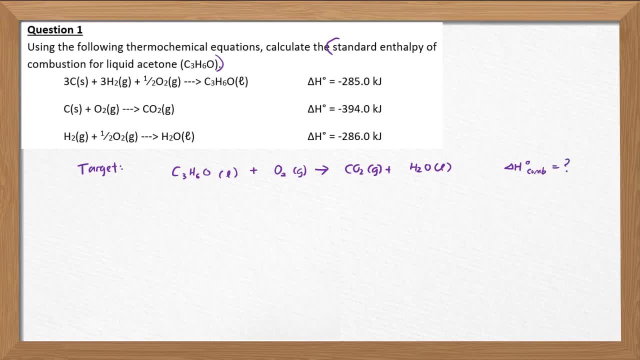 combustions. so balance up your equations: c3, h6o, we keep it one mole, so we have three mole of carbon dioxide, we have three mole of h2o and we have nine over two mole of oxygen gas. so this is our target equations based on, based on the questions of what we want to find all right. 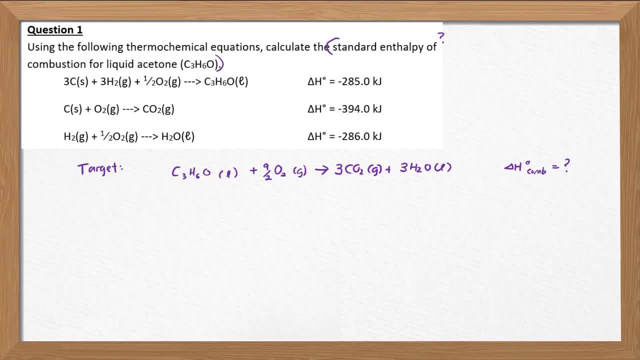 so according to the, the, the equations enthalpy. so according to the formula, the enthalpy of combustions or enthalpy of reactions equals to the total enthalpy of formations of the product minus the total enthalpy of formations for the reactant. so we need to write in specific together. 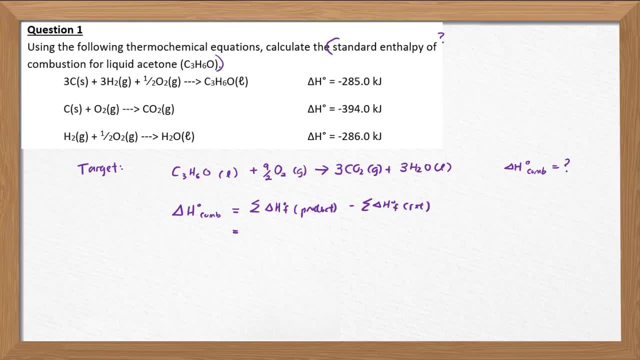 with the stoichiometric ratio. so for product we have three mole of carbon dioxide, so three times the enthalpy of carbon dioxide plus three times the enthalpy of formations for h2o. so all of these are the product. okay, all of these are the products and minus the reactants, so we need to minus. 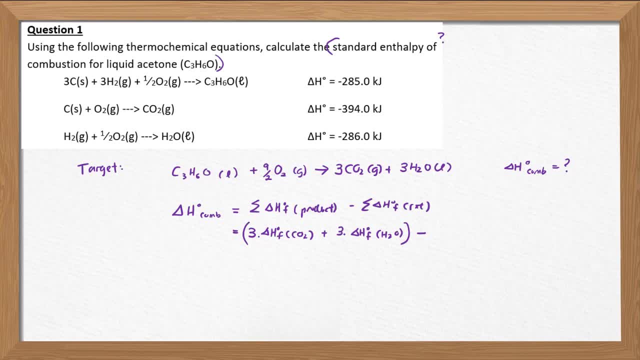 one times the enthalpy of formations for c3h6o and also the enthalpy of formations of the oxygen, but turn our energy back to the squared value. lets consider this скажем for other ways we miss the r? dichro Overto times the enthalpy of formations for oxygen gas. 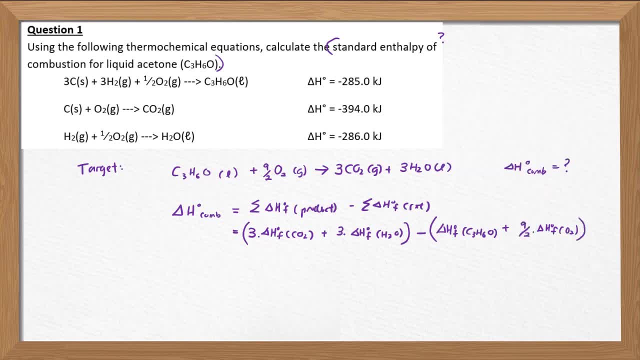 remember that the enthalpy of formations for oxygen- because oxygen is the element, therefore enthalpy of formation, so oxygen is element of the body. Therefore enthalpy of formations for oxygens equals to zero. Let's substitute with the value, So three times- enthalpy of formations for carbon dioxide is negative, 394.. 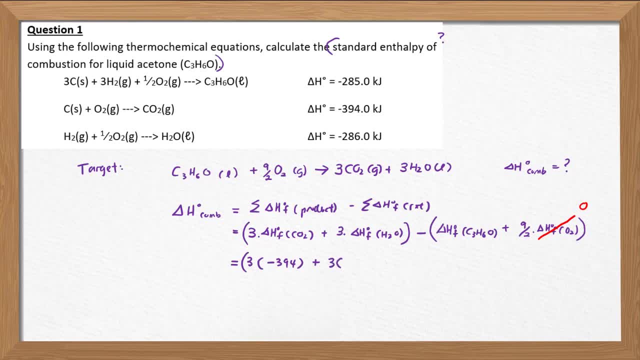 The enthalpy of water: three times negative: 286, minus the enthalpy of acetone, which is negative, 285.. And finally, to find the enthalpy of combustion, it's equals to negative 1755 kilojoules per mole. 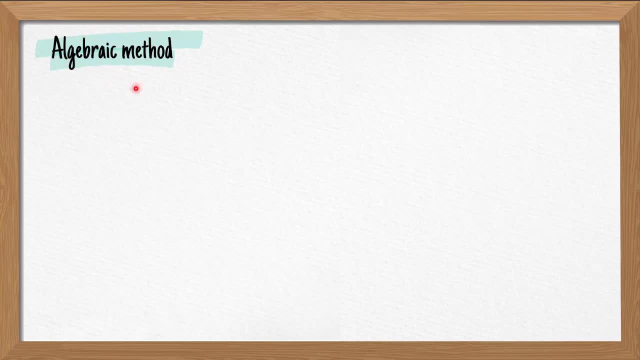 All right. so next let's look at algebraic methods. So for our algebraic method also, first we need to identify the target equations. Remember that target equation is the one that we want to answer, we want to find. So use the definitions of enthalpy to construct the equations needed. 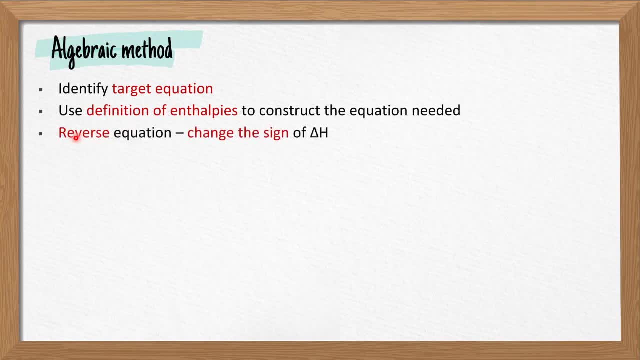 And if you want to change the signs of delta H, you need to reverse the equations. So when reversing the equations you change the sign at the same time. And if you want to change the stoichiometry, so that means if the equations, you need to multiply with two. 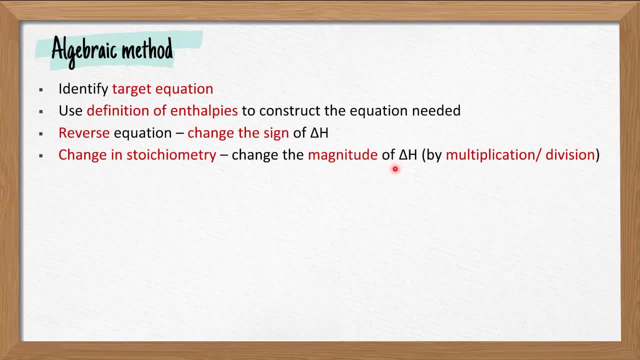 then you need to change. And if you want to change the magnitude of your delta H by either multiplications or divisions. So for example, if you want to multiply the whole equations with two, the delta H also you need to multiply with two. 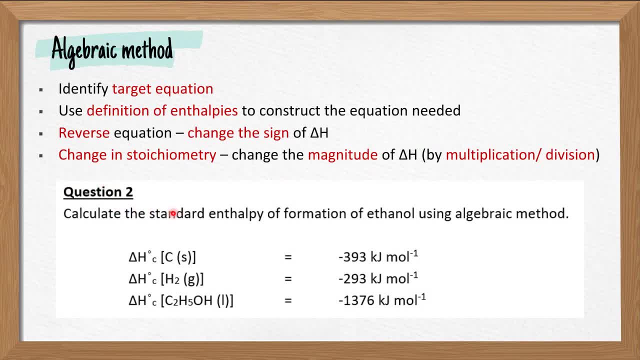 So in question number two calculate the standard enthalpy of formations of ethanol using algebraic methods. So you are given enthalpy of combustions- carbon, enthalpy of combustions- hydrogen, and enthalpy of combustions for ethanol. 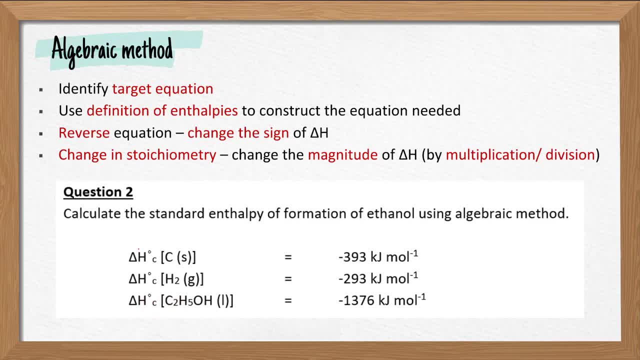 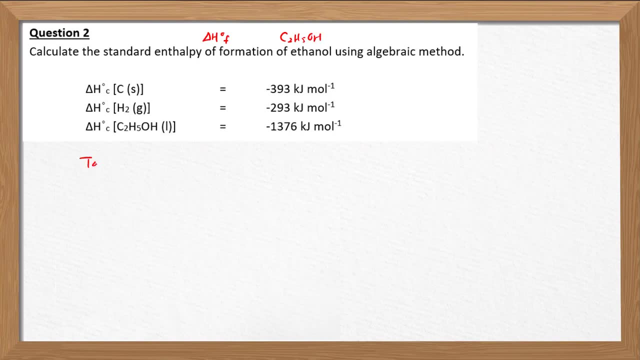 So in this case, our target is to find the standard enthalpy of formations for ethanol. Alright, you need to find a balanced equation for this target, Alright? so first of all, let's look at your target equations. So, enthalpy of formations, first definition. it says that when one of the two equations is equal to one, the other one is equal to one. So, for example, if you want to find the standard enthalpy of formations for ethanol, you need to find the standard enthalpy of formations for ethanol. 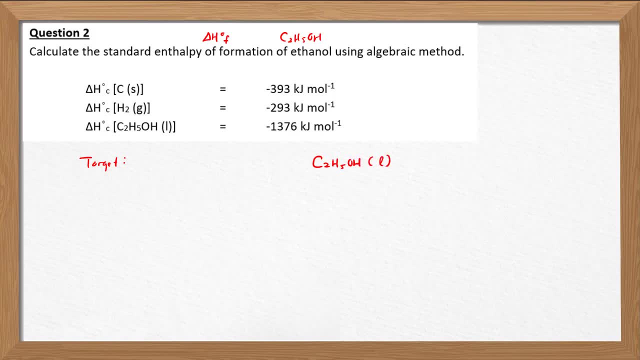 So here the same thing happens. One more of the compound is formed. So in this case our compound is ethanol. Keep this ethanol one more. So in this formula you can see carbon hydrogen oxygen. So that means the elements must have carbon hydrogen and oxygen. 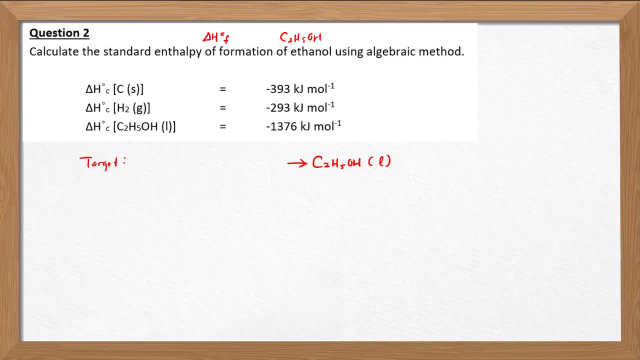 So when one more of the compound is formed from its element under standard state. So carbon standard state is solid Hydrogen Standard state is solid gas. in H2 and oxygen, the standard state is at O2 gas. All right, so once you've identified the 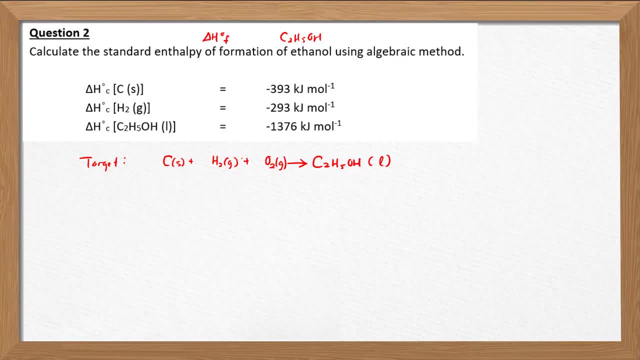 element. the next step is to balance the equations. Remember to keep the ethanol as one mole, as that is our focus. So we balance out. we have two mole of carbon, we have three mole of H2, we have half mole of O2, as there's only one oxygen on the right hand side, So half of the O2 it live with only one. 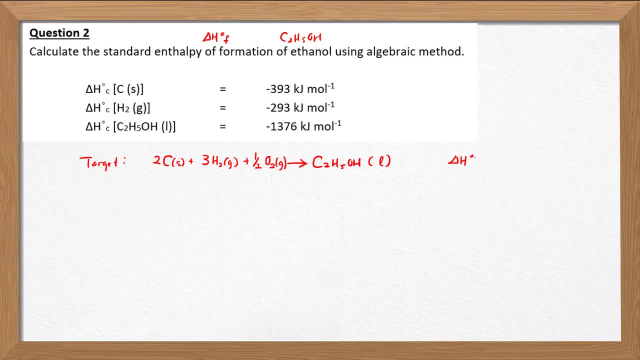 O. And then we want to find this enthalpy of formation. All right, so next one, we want to look at this information: enthalpy of combustions. So recall back the definitions of combustions. So burning carbon in oxygen produce carbon dioxide gas. So the equation is already balanced. then we 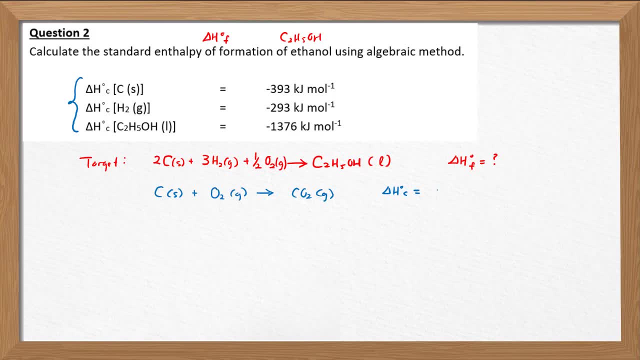 write off The enthalpy of combustions, negative: 393 kilojoule per mole. So the second one, enthalpy of combustions for H2.. So when one mole of hydrogen is combusted in oxygens, they're producing H2O. 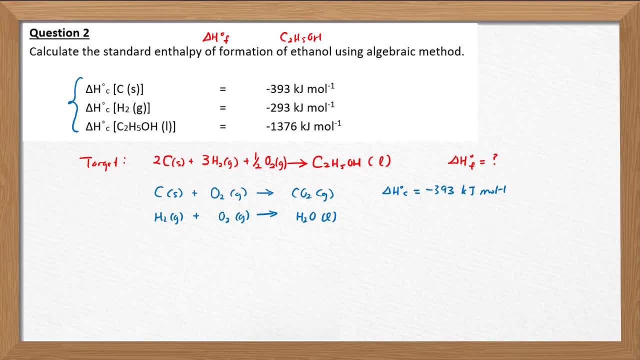 liquid. Okay, because you only got hydrogen and oxygen. so you're producing H2O. So balance up your equations. you've got half mole of the O2.. Make sure you keep carbon, you keep H2O, you keep your time. So we write the enthalpy negative: 293 kilojoule per mole. 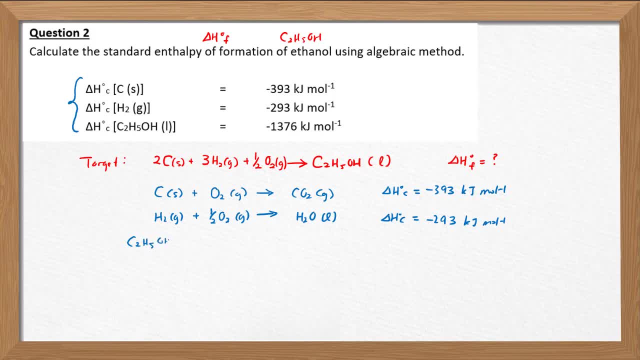 All right, the last equations. So when one mole of the H2 is combusted in oxygen, they're producing carbon dioxide and water. So the enthalpy of combustion is negative, 1376 kilojoule per mole. So balance up the equations. keep this ethanol one mole. We have two mole of carbon dioxide, 10,. 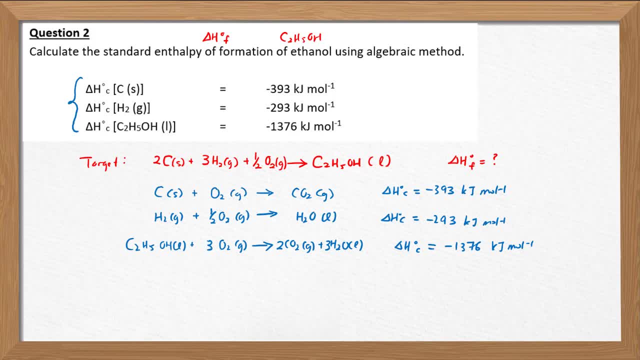 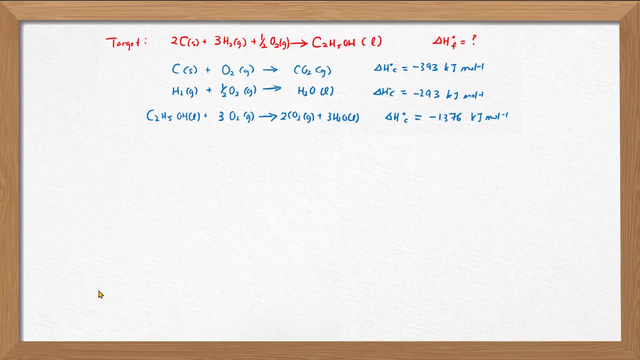 three moles of hydrogen And three moles of water. we have three moles of oxygen on the left hand side. All right, so the reasons why we have our targets is we need to solve all these equations. So after we can solve the unnecessary species, we will get back the target equations. Okay, so here, if you look, 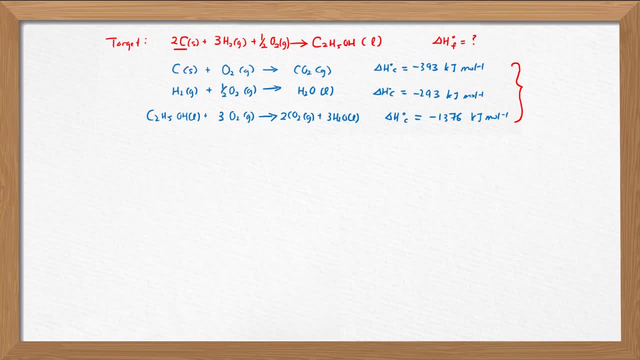 at the target we have two c. So that means in the first equations, the enthalpy of combustions for carbon, we need to multiply with two. okay, we need to multiply with two for the whole equations, including the enthalpy, and then after that we look at this hydrogen in our target we have three. 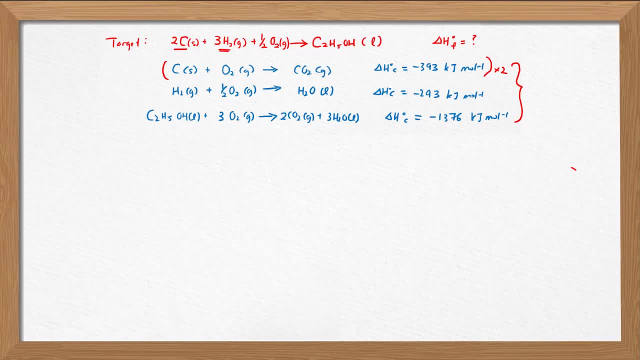 molecules of H2. therefore, for the second equations, for the enthalpy of combustions of H2, we need to multiply with three and the next one is the enthalpy of combustion. as you can see over target equations here on the right hand side, that means for the equation enthalpy of: 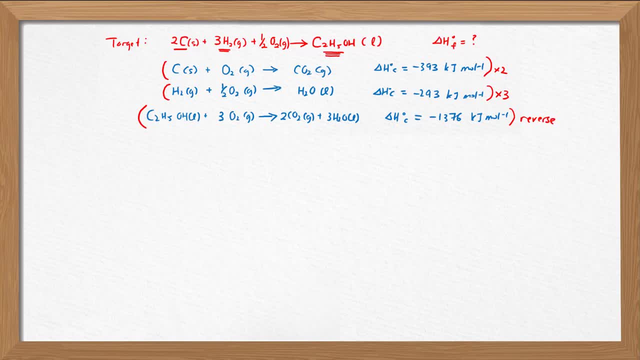 combustion. we need to reverse it so that we can get the ethanol at the product side. so we reverse the whole equations to make ethanol as the product. so as you do this one, the enthalpy of combustions for this species. we need to reverse it so for negative sign it will become positive. 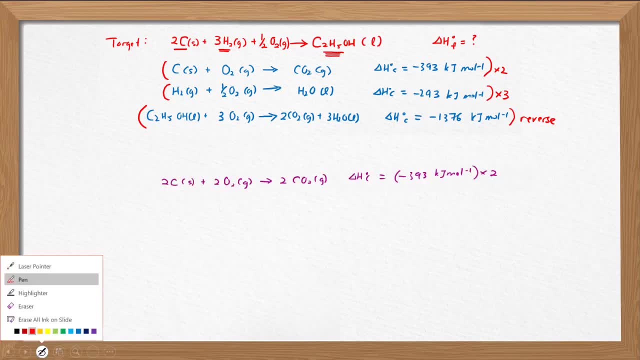 sign. so after we solve this, you 2c plus 202 to produce two carbon, carbon dioxide. so the enthalpy times with two. so I leave it like this, first to see that, okay, I have already multiplied with two in this case. then the second equation: 3H2, 3 over 202 to produce 3H2O, enthalpy times with three. and the last one we 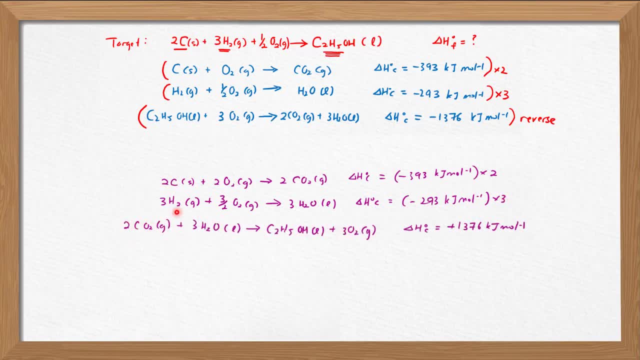 reverse the whole equations to become 2CO2- okay, change the positions- and then 3H2O and to produce one mole of ethanol and three moles of oxygens. so the enthalpy of combustions will reverse the sign from negative to positive. and after you have got all these, 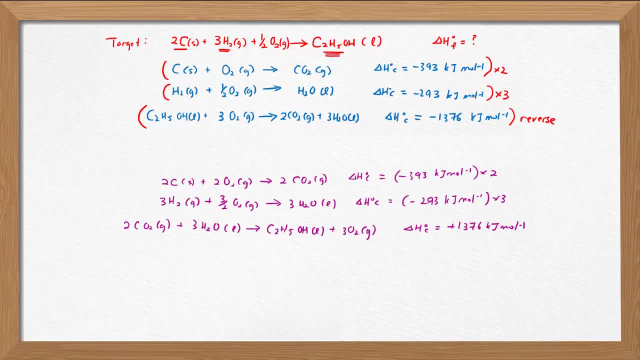 equations solved. so now we want to see whether which species we can cancel off. so, first of all, carbon dioxide- we can cancel off, 3H2O we can cancel off and the oxygen- we are having this one. we are having this one which is carbon dioxide, and this one is carbon dioxide and this one. we want to see what happens. 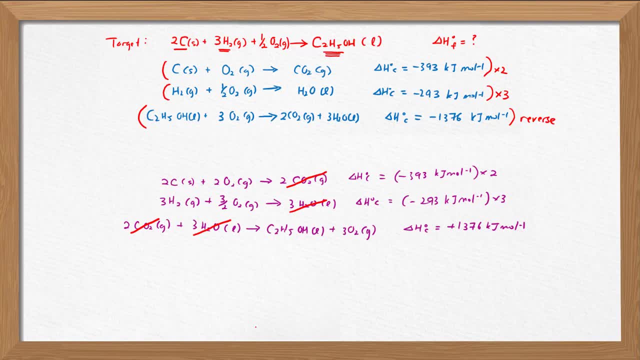 if we change the equation- so let's take a look at this one- we can see that if we change the equation, so that's x2. so could you see the difference in this equation, where xs, u, o is equal toero2 and eO 2 are all equal to 0. 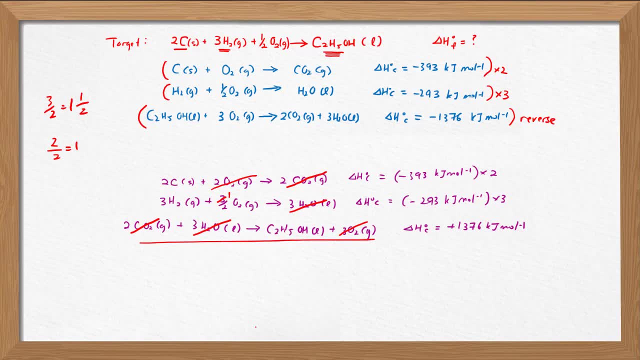 then you need to write down, rewrite the equations. whichever species that left, You can see over here. after you're cancelling the unnecessary species, you left with 2C, 3H2O, half-oxygens and ethanol, which is the same as the target equations that we have written earlier. 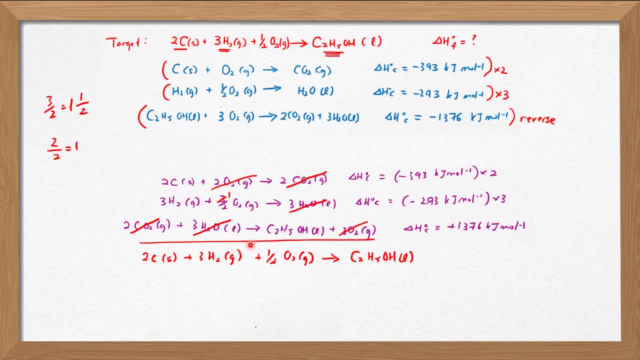 Alright, so after you have got these target equations, we just add up all the enthalpy of convulsions here. Okay, we add up only To get the final answer: MW of formations negative: 289 kJ per mole. 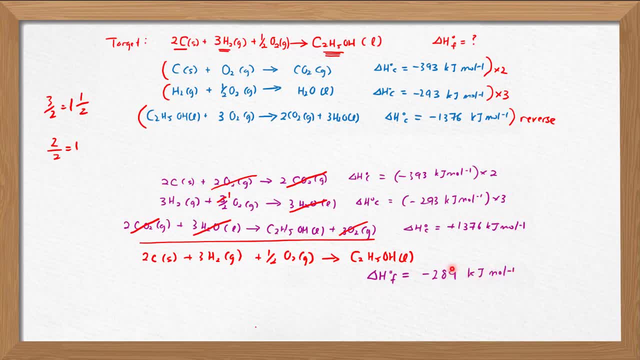 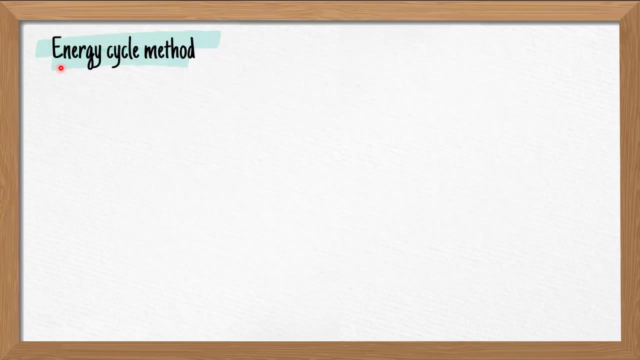 Again, this per mole refers to when one mole of the ethanol is formed. this much of energy is released. Okay, 289 kJ of energy is released, So per mole refers to one mole of ethanol. Alright, so the last method we have here is energy cycle method. 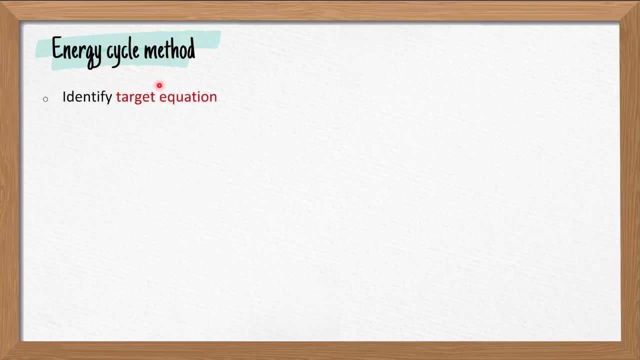 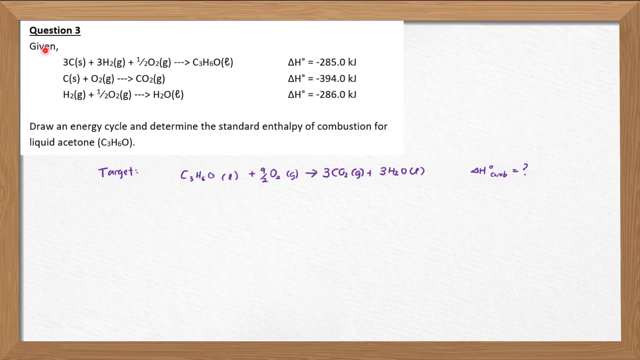 So for energy cycle method also, we need to identify what is your target equations. Again, target is what we want to find in the questions. So use enthalpy to construct equations needed. Take notes at the directions of the arrow In this example, questions 3, the questions is slightly the same as questions number 1.. 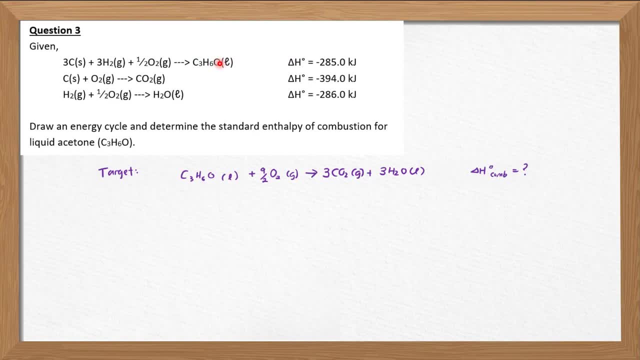 So you have the enthalpy of formations for C3H6O, the enthalpy of formations for carbon dioxide, but you need to find the energy cycle method. So for energy cycle method also, we need to identify what is your target equations. 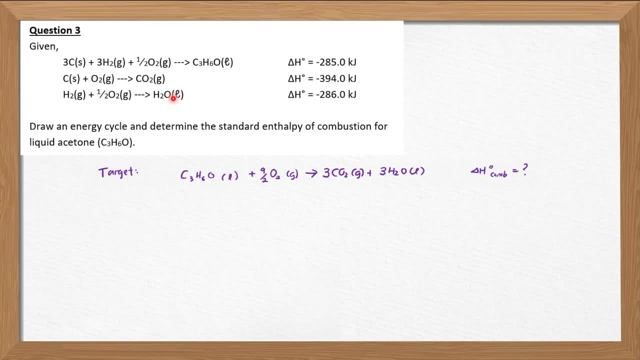 enthalpy of formations for H2O. So again, revise, back again. Formations say that when one mole of the compound is formed from its element, element, element at their standard state and the standard condition. So in this case you need to draw an energy cycle and determine the standard enthalpy. 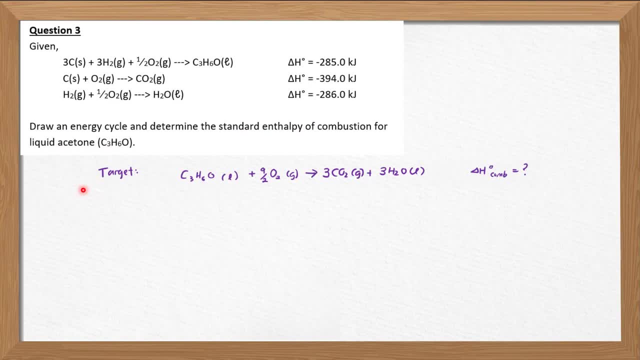 of combustions for liquid acetone. So you can see that similar, like in your questions number one, or similar as questions number one, in which you use the formula. In this case we want to see, using the same questions, how are you going to solve it using energy cycle? So again, target is: 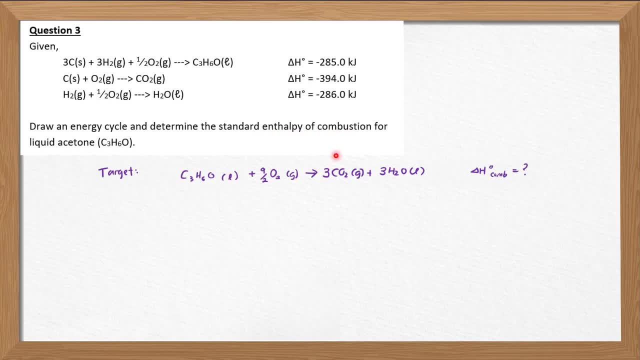 the enthalpy, the standard enthalpy of combustions. When one mole of C3H6O is combusted, heat is released. So the following equations- you need to complete it, Okay- O2, and then product is carbon outside. 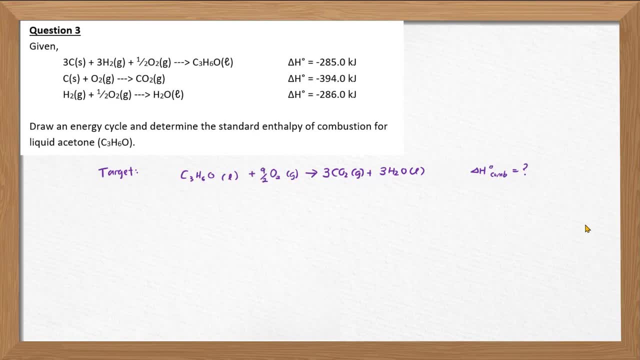 And H2O and then balance your equation. Okay, so you can start off using this target equations. you can see C3H6O, you can see carbon dioxide, you can see water, So I choose the easier one to start off. I think that the second equations is simple, So I start off with carbon, carbon dioxide. So as 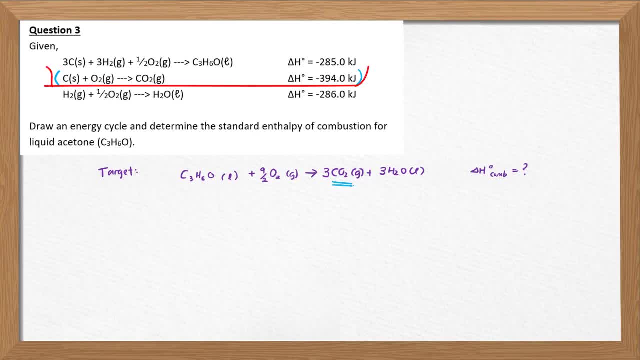 you can see over here, we have carbon dioxide as the product in that equations here. All right, so that's it. That means I will produce the product from carbon solid and oxygen gas. Okay, so, as you check it back again, carbon plus oxygen to produce carbon dioxide, But in this case, because our target 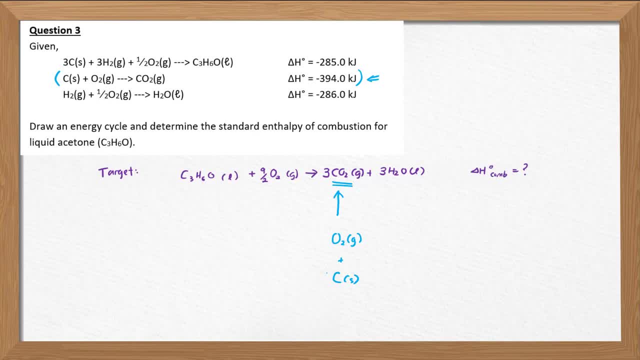 equations. we have three molecule of CO2.. Therefore, I need to have three carbon. I need to have three moles of oxygen. So this equation is not our standard math variance. When you have an aggrav, Madonna, Just compare your answer: inconsistencies. 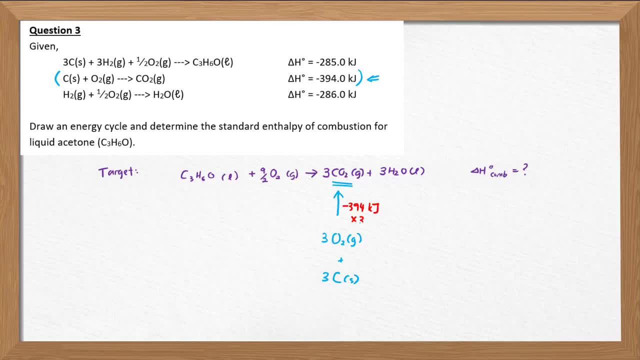 using the equation, And here you will find that C3H6O and then cold, you have H2O plus oxygen leaves in that equation. so it's either C3H6O or you have H2O plus oxygen here. But actually 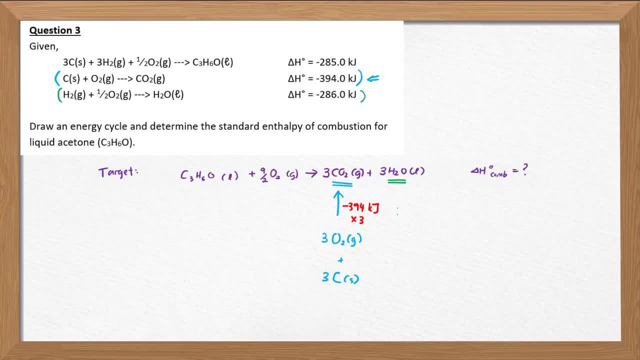 if I think about the 가는 Kanye driver's equation, all I need is C3H6O plus H2O plus 16. friend, were that answer Here you have False. That's not the math answer. Still, Because's not verdade. Father called 삼성 and now you do you yourself from eternal mass and values of mu and takes different scripture. because the球 reacting you with nutrients there will be am repeated for the water. so that means our enthalpy over here. negative 39 for kilojou. we need to multiply with three times. 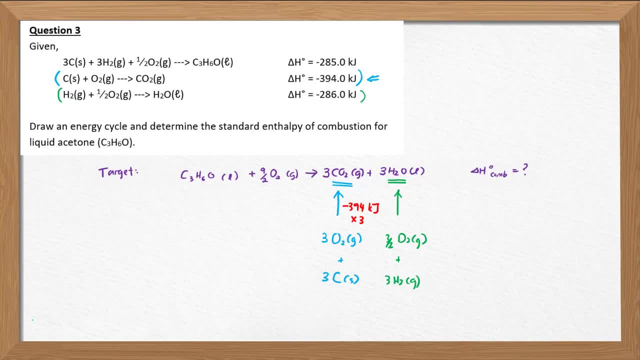 moles of oxygen gas, The enthalpy negative 286 kilojoule. we multiply with 3. also Okay, we multiply with 3 because the equation over here is only 1 mole of H2O. Here we have 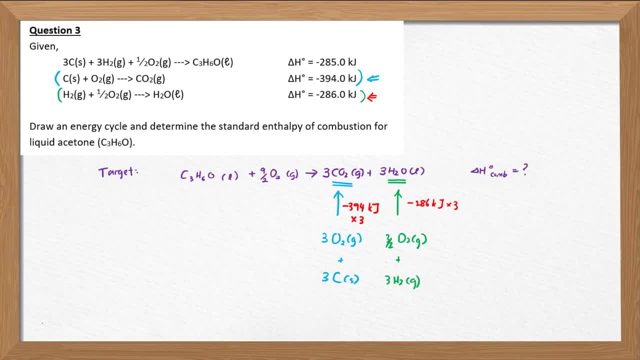 3 moles, so we need to multiply with 3.. Alright, so the last equation, the first one, carbon hydrogen oxygen, to produce 1 mole of C3H6.. So, as you can see where madam underline, 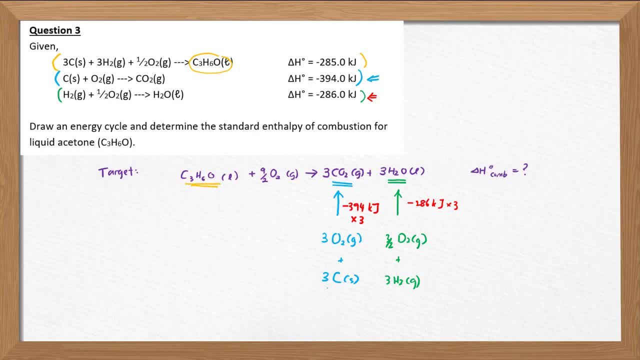 C3H6 as the product. we have 3 carbon, we have 3 H2O. So what is missing over here? we just add on 1 over 2 oxygen gas to produce the product C3H6O- your acetone. Okay. so we check it again. 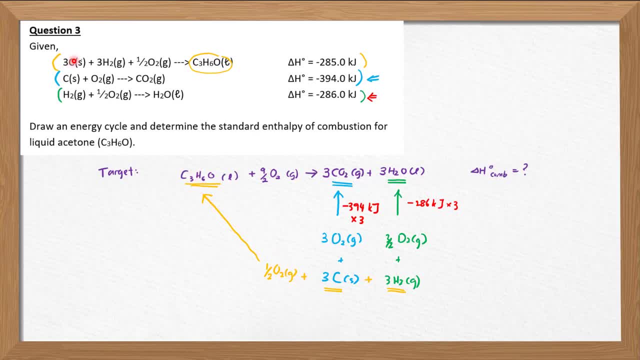 Okay, check it again using the first formula here: 3 carbon, 3 H2, half O2,, 3 H2, 3 carbon, half O2- to produce 1 mole of acetone And for this equation value which is equal to negative 285. 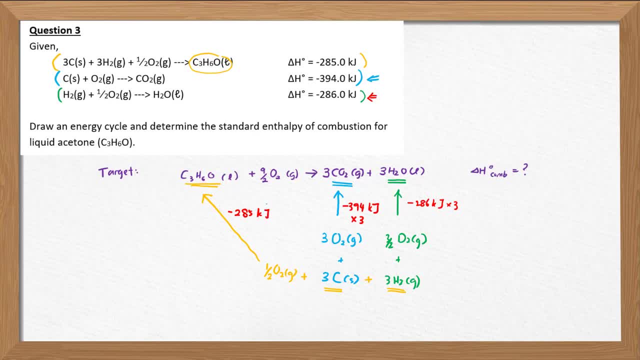 kilojoule, Okay, without reverse, without multiplying anything, so negative: 285 kilojoule, Okay. so now I want you to look at this diagram. So I represent the arrow using color, following the using the equation here. So for our target equation we want to find the entropy of: 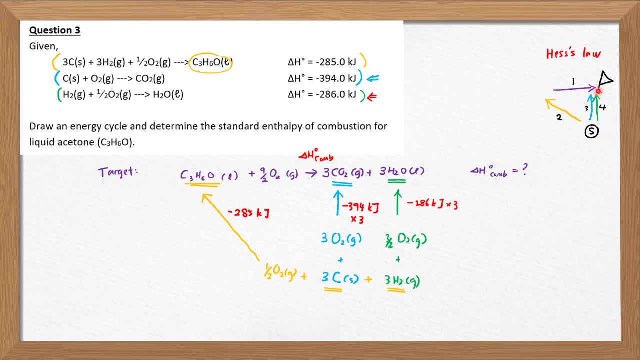 combustion. So it's in the directions like this: Okay, from the left to the right, And then the blue and the green color. they are heading to the same directions. And then for number two is: from this point until this point. Okay, so in Hess's law, the single set referred to here, this S. 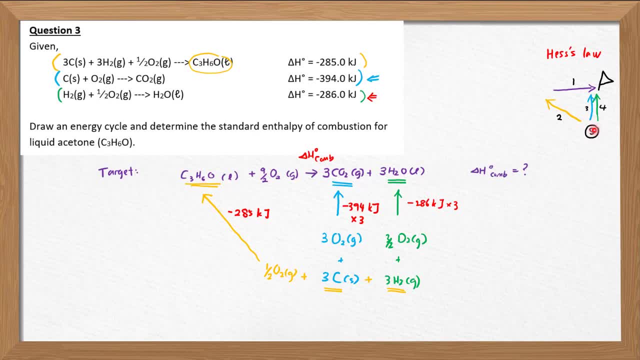 madam, put it as the starting point, Okay, and then you see the starting point in just one step. reaching the end point, Okay, reaching the finishing point. and then, if i want to do in a multiple series of steps, okay. i'm following the arrow number two, following the number arrow number three, so, as you can see over, 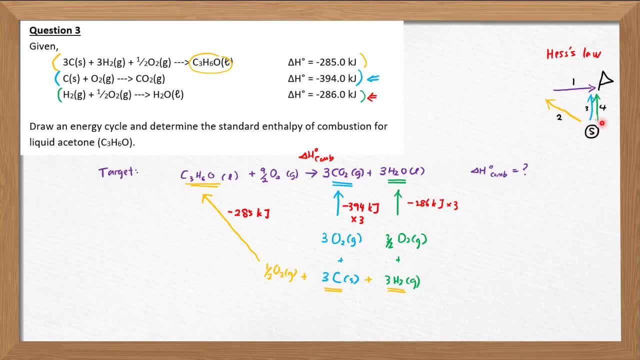 here: uh, two, three, four: the arrow starting from the same point and then the rest of the arrow that stop at the same point. this point doesn't have stop point because, um, from starting you proceed until this elbow and then you will still continue until you're reaching the finishing point. 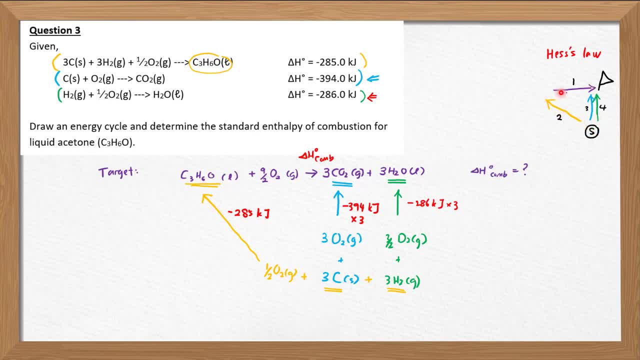 so this is a single step. this is a multiple series of steps. so if you want to look at this, you will see the direction: single step and multiple series of steps. so now we want to construct a formula based on your energy cycle. so that means three and four is equals to one and two. 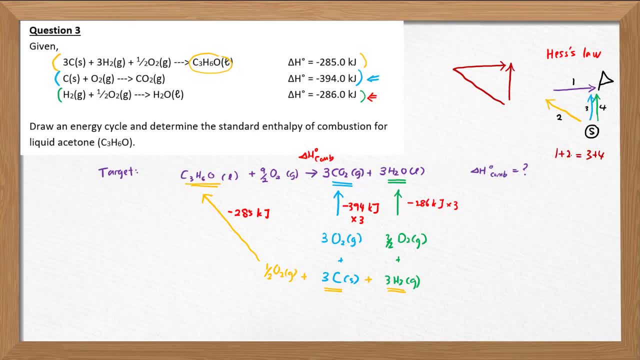 okay, a single step is the same as the- uh enthalpy change for a multiple series of steps. okay, so three and four is over here. one and two is over here. so now we want to make our equation based on the diagram that we formed, so i label this one. 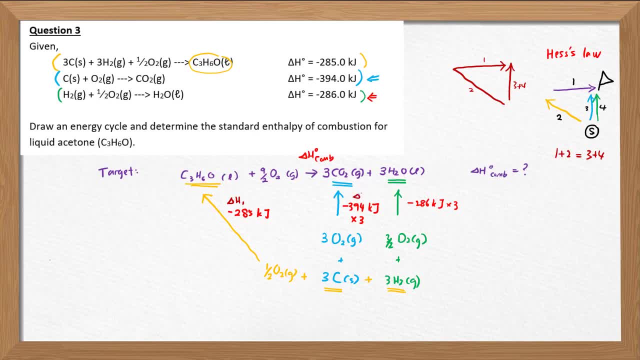 is the enthalpy one, and that'll be two, and that'll be three to make my equation. so, and that'll be one, one, and that'll be two and that'll be three to make my equation. so that's the second end of the equation that i'm gonna write down, and then i'm gonna multiply this one. so this is the second step. 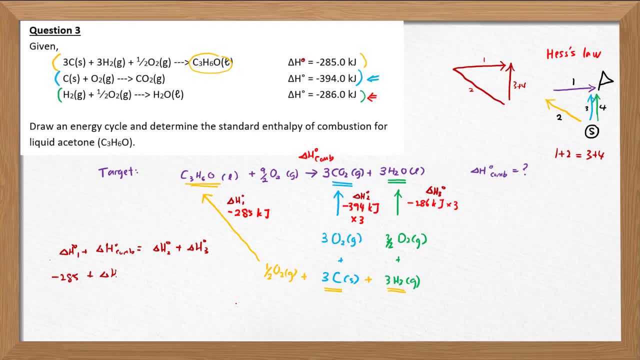 here and, as i'm gonna bring my equation here, we are gonna have the equation equal to one and two plus the second, and thou be plus the third and healthy. okay, don't forget that in the question is give you standard. so the the following enthalpy: we put it as standard condition.